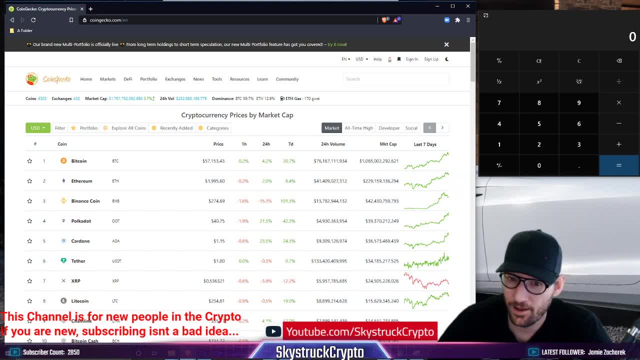 Ethereum, which means, if Ethereum is a competitor to Bitcoin, then what if this $40, it ends up being $57,000, right? I've also heard Cardano is a competitor to Ethereum, right? So what if this $1 went to $57,000?? Why would I buy a Bitcoin or Ethereum if I? 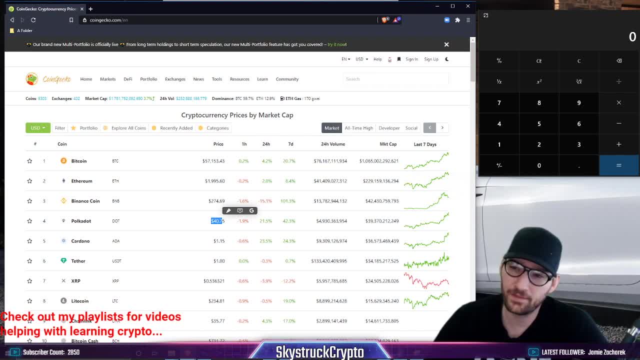 this is a much better opportunity, right? And that's fine. to think that way, I mean don't. I mean not, it's not fine. I guess we need to rethink the way we think things, because the price is completely irrelevant when it comes to crypto. All right, In order for $40. 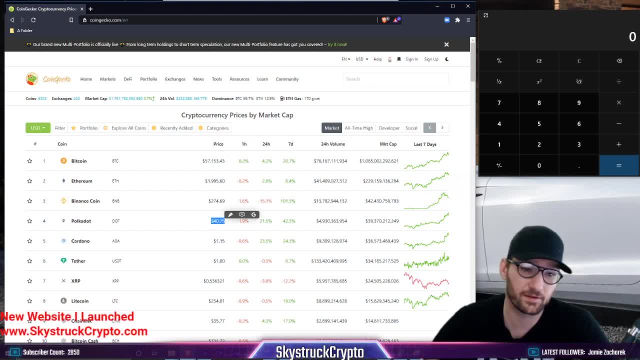 to get to $57,000, it's it is- is this coin would be way bigger than Bitcoin would ever be- or not ever, but it would be right now, And I'll show you what I mean in a minute. but it's not about the coin price, It's about the current total market. 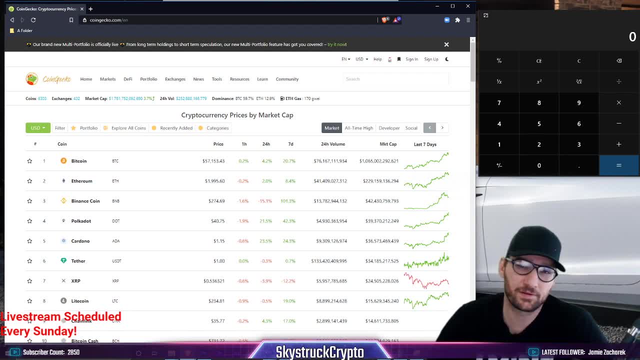 cap of the company. Now here is where a misconception also comes in. People think that they need to buy an entire Bitcoin, right? Gene Simmons recently posted that he liked Cardano because it's easier to buy Cardano than it would be Bitcoin, Not knowing that Bitcoin has a lower 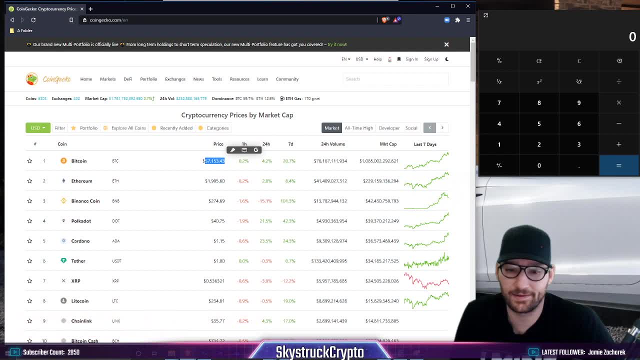 denomination of a of a called a Satoshi. You know it's like a, you know like a hundred dollar bill to a penny, right, It's like you can't say like, well, not everyone could get a hundred. dollar bill. but it's like dude, you can get spare change And you you still have that. you know that dollar amount in Fiat. you know it's different anyways, But the price is completely irrelevant. right, You can put $10 in Ethereum. you can put $5. 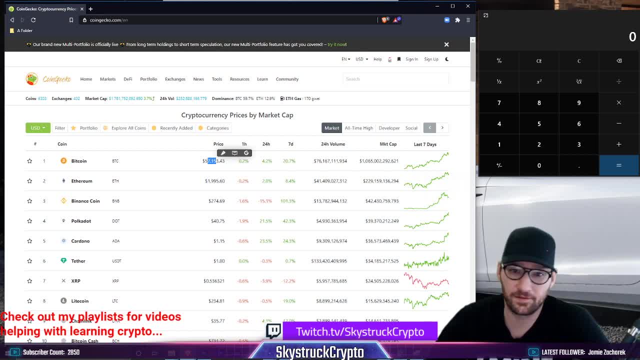 into Bitcoin. You can put, you know, you can put- 10 cents into Bitcoin, right, That's the point of these cryptocurrencies. right, You can be able to hold a very, very, very small, minuscule amount and be able to transfer and trade that small amount as well. But let me 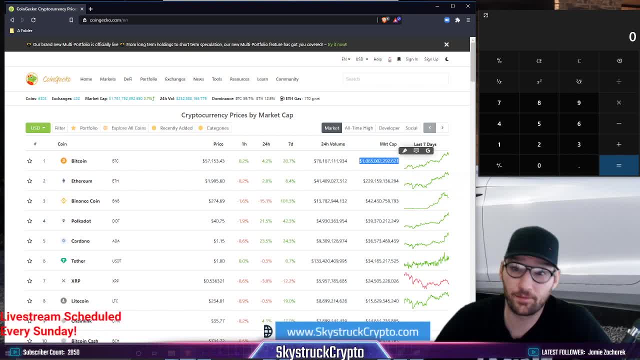 share with you what really matters, And that's right here: the market cap. This is what really matters. So, when people say, what if Ethereum got as big as Bitcoin, right 2000,. and this is going to be over, you know. 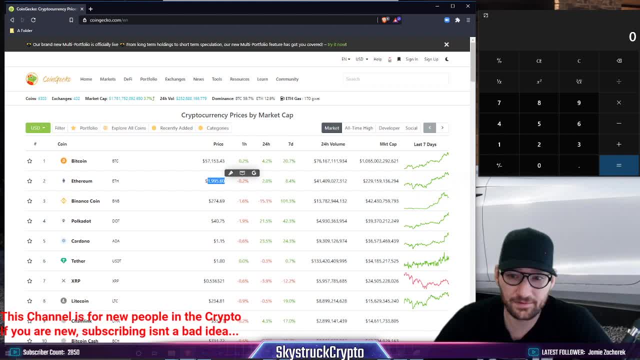 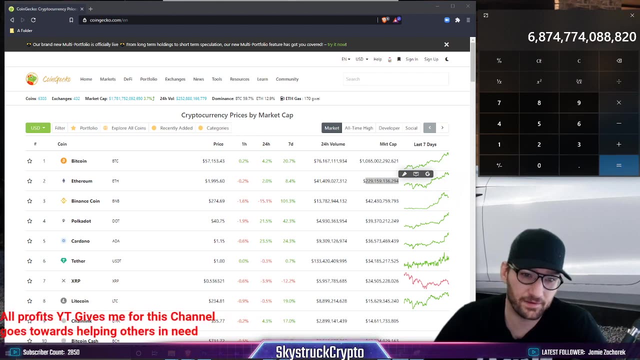 30X. Well, if it went to a 30X, that means it would hit a two. you know, $230 billion market cap times 30, right? So essentially what you're saying is: um that it that if if Ethereum uh hit the same price as Bitcoin, Ethereum would be at Bitcoin's current price. Ethereum would be almost seven times bigger than Bitcoin currently, because you need to always look at the market cap. This is what shows the worth of the company. Now why is the coin price different? That? 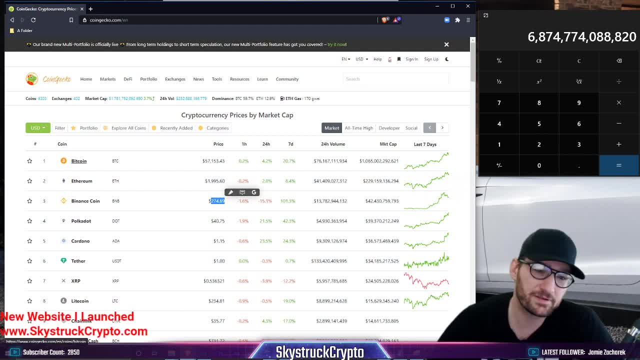 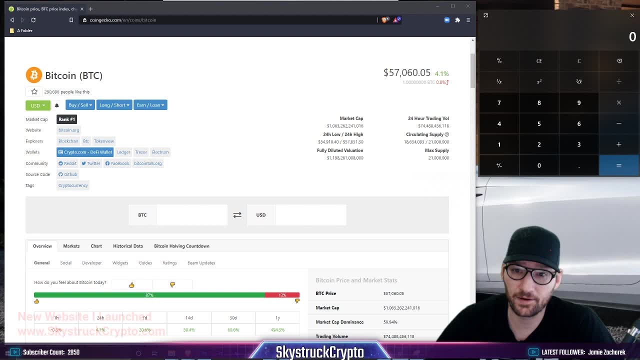 is because the circulating supply. So let's go into Bitcoin, for an, for example. So Bitcoin's price is $57,060.. Okay, The market cap is a little over a trillion, The circulating supply is the 18,634,093.. 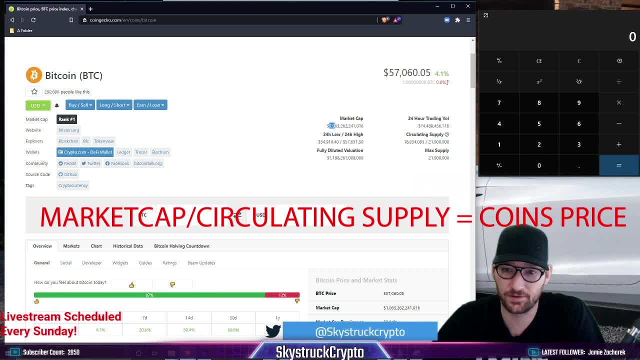 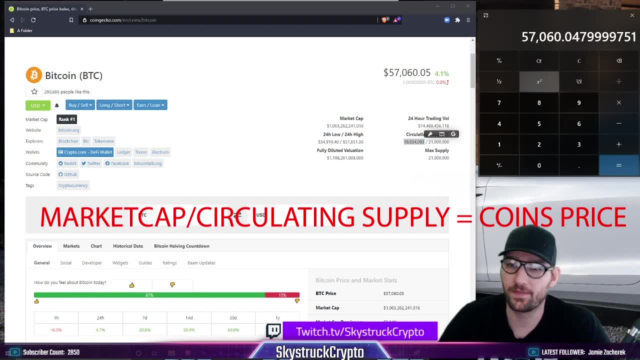 So if I were to take the current market cap, which is that trillion dollars, and I were to divide it by the circulating supply, then I would get the current price of Bitcoin $57,060.. And uh, the price is a little bit skewed at the pennies, but uh, you get the picture. 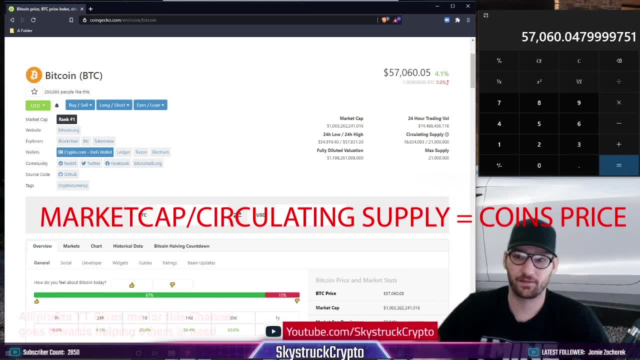 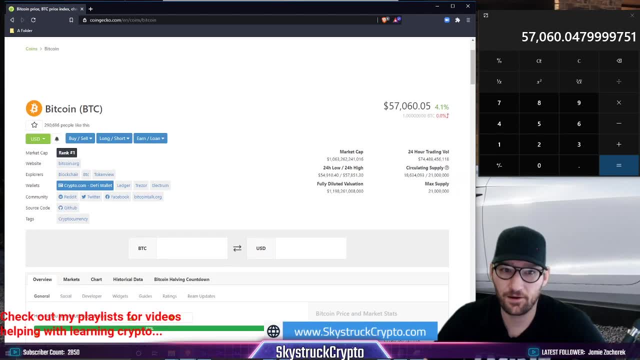 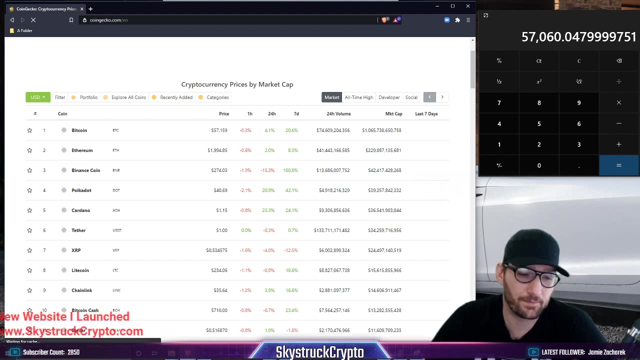 right. By different exchanges, the price fluctuates and everything like that, because the circulating supply is always constantly changing and um, but you get the picture. that's how you get the price. So this is what you need to look at: market cap every single time. Now, if now a big conversation. that people are having right now is: what if Polkadot? you know, Polkadot is a competitor Ethereum and I think they are when it comes to market cap for sure. Um, and they are currently at a $40 billion market cap. 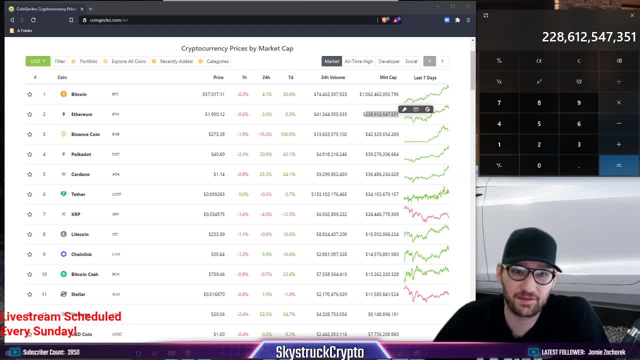 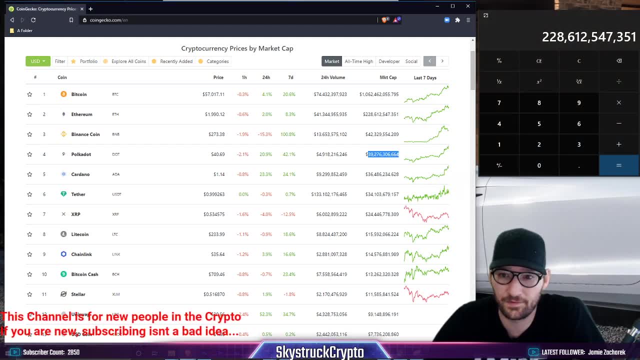 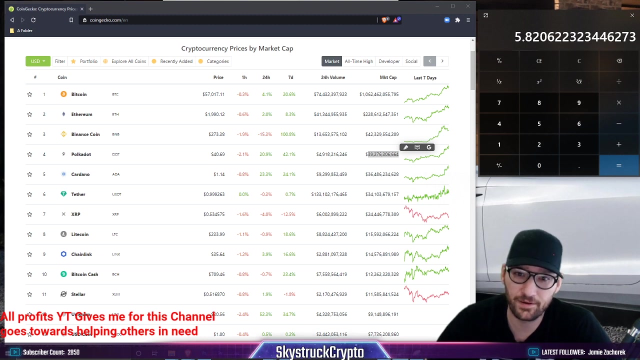 So if Polkadot got to be as big as Ethereum current price, we would have to take the current price of Ethereum and divided by the current price of Polkadot, and that equals 5.8.. So, essentially, if Polkadot got to be as big as Ethereum, then we would have to take 5.8. 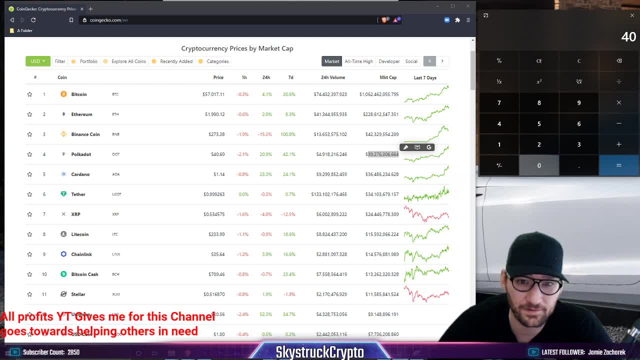 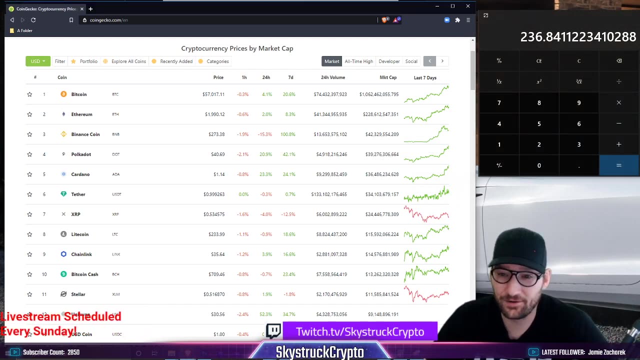 and times it by the current price, times $40.60.. So if Polkadot got to be as big as Ethereum, at its current price, it would be a $236 coin. So when you were looking at a coins price, for example Cardano, it would be pretty much. 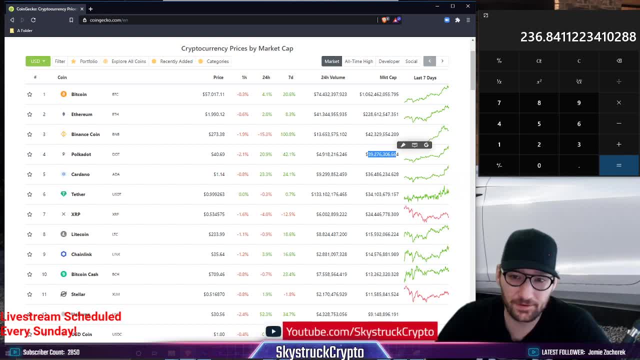 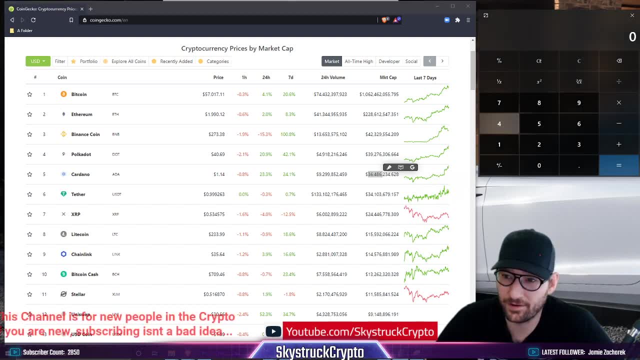 the same thing. Uh, Polkadot is around $39 billion. market cap Cardano is 36 billion. So, uh, you would have to take that dollar 1.14 and times it by 5.8.. So if Cardano got to be at as big as Ethereum at its current price, um, then it would be.